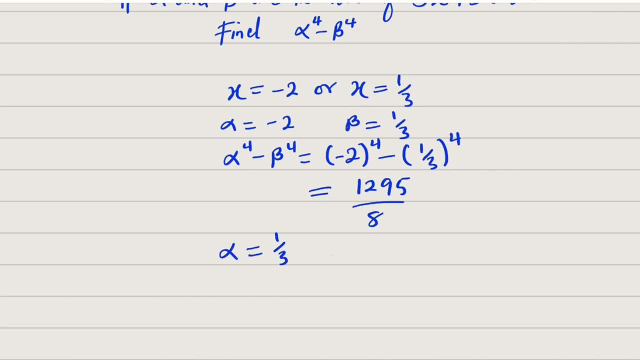 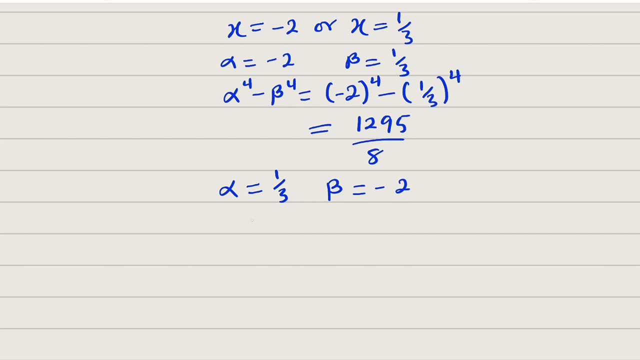 alpha is equal to this 1 over 3, and beta equals negative 2.. The same thing: if you say alpha to the power of 4 minus beta to the power of 4, this will be equal to 1 over 3 raised to the power of 4, minus negative 2 raised to the power of 4.. And you shall obtain negative. 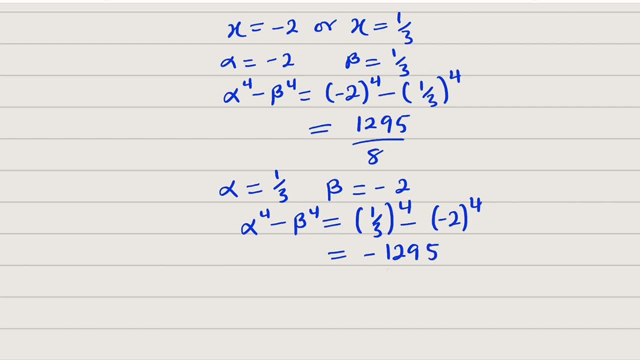 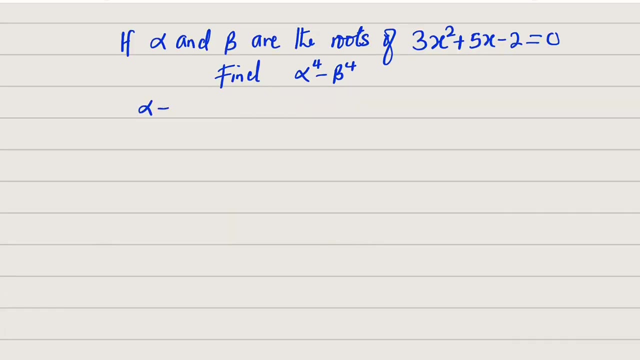 14 fragile billion thousand two hundred and ninety five divided by 81. all right, this is 81, sorry. so this are the two possible solutions. now let us start working on that. you know that alpha plus beta, which is sum of roots, can be often by taking negative 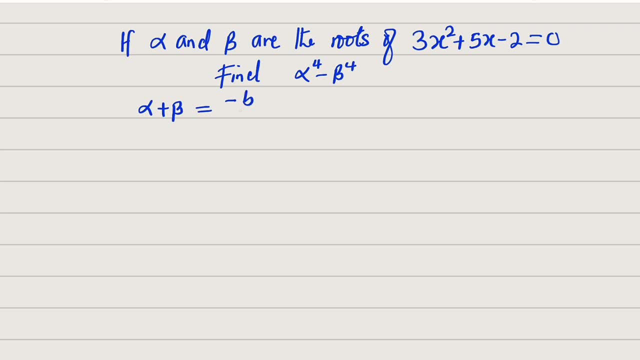 the coefficient of the middle term, which is X, divided by the leading coefficient, which is a, and this is equal to. you know, B is going to be equal to 5, but this is negative. so we have negative 5 divided by a, which is the leading coefficient. 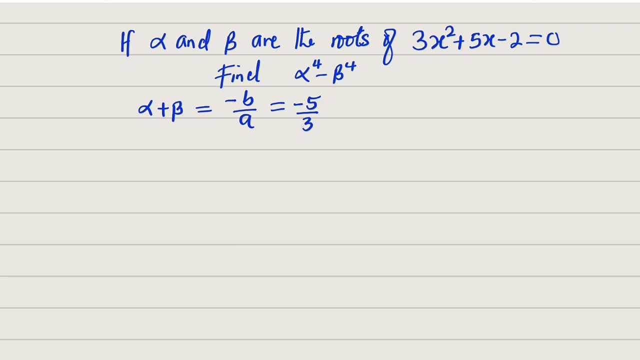 which is 3 here. so we have 3. so this is the sum of roots. let us find a product. the product will be alpha x, beta, which is equal to C divided by a, and you know that C is the constant which we have as negative 2, and A is the leading coefficient, which is 3.. Now we 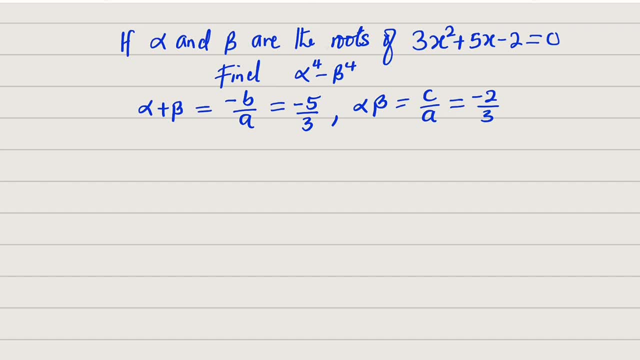 have our product, which is negative, 2 over 3.. Now let us simplify: alpha to the power of 4 minus beta to the power of 4.. Alpha to the power of 4 minus beta to the power of 4 can be simplified as alpha squared minus beta squared. 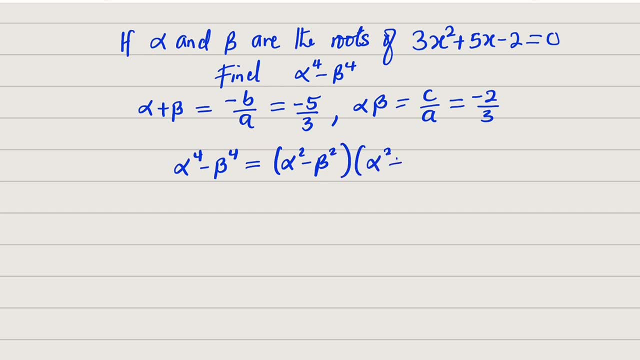 multiplied by alpha squared plus beta squared. If you expand this you shall get this back. But this is also difference of 2 squared, which can be simplified as alpha minus beta, multiplied by alpha plus beta, and we have the other one, alpha squared plus beta squared. Remember, in our simplification we only have alpha plus. 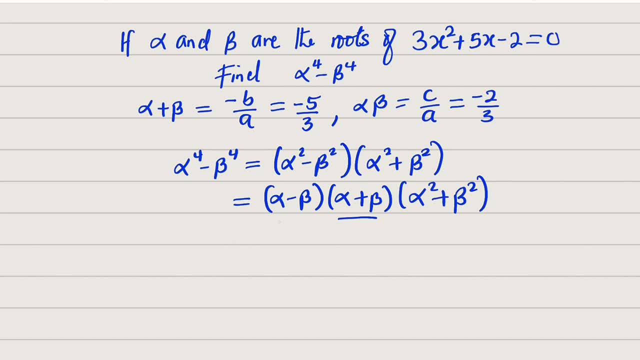 beta and alpha multiplied by beta. Therefore, we have to also simplify this and this, Let me start with this one- To obtain that you can expand alpha plus beta to the power of 2, which can be written as alpha squared plus beta, squared plus 2 alpha beta. This is exactly what we are looking. 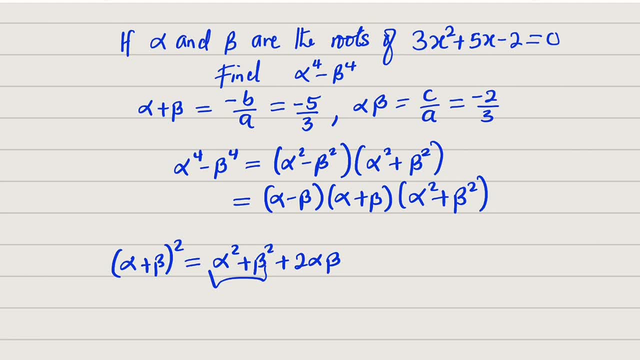 for You can see it here. We can now make it the subject of this equation. It will be equal to alpha squared plus beta squared equals. you take this: you subtract this alpha plus beta to the power of 2 minus 2 alpha beta. now you can write this instead of this: 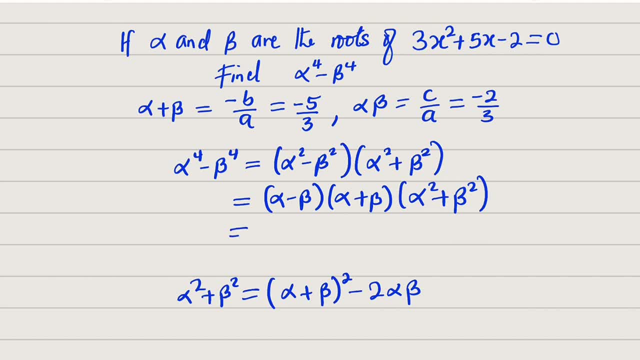 all right, let's continue. so this becomes alpha minus beta multiplied by alpha plus beta, then multiply by. we have all of this alpha plus beta squared minus 2 alpha beta. now you can see. we have sum here. we have product here. we have product on this class d. 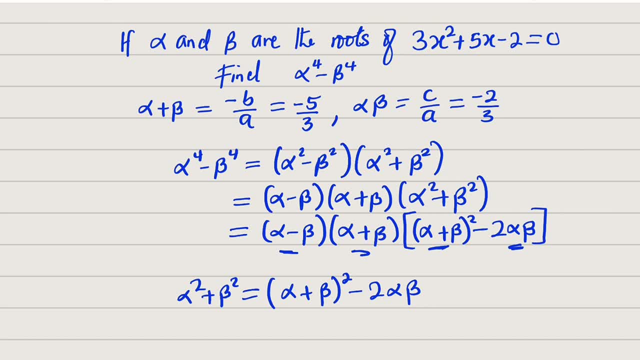 sum here. This is only what we have to simplify. again, To simplify that, we need to expand alpha minus beta squared, and this is equal to alpha squared plus beta squared. then minus 2 alpha beta, Again, alpha squared plus beta squared is just equal to this, because that's what we 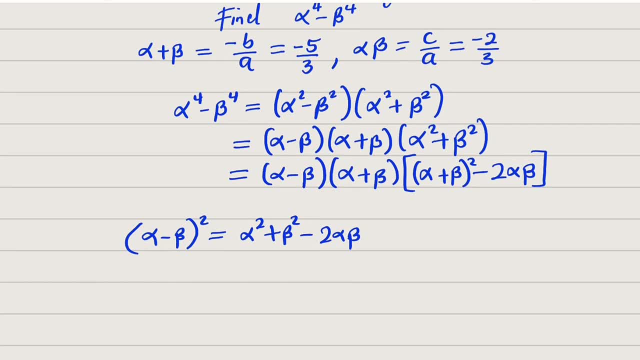 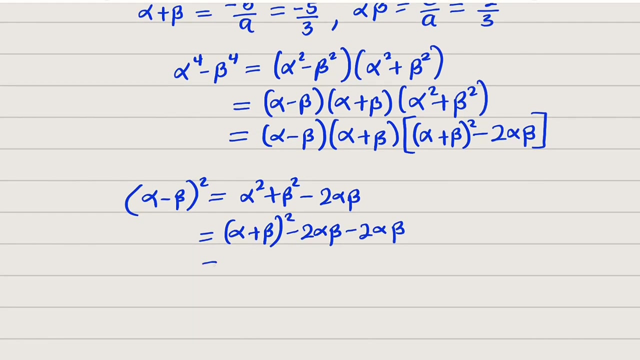 simplify to get that. So this is equal to alpha plus beta, to the power of 2 minus 2 alpha beta. but we have another negative 2 alpha beta, negative 2 alpha beta here, making negative 4 alpha beta. this is equal to alpha plus beta, squared minus 4 alpha beta. 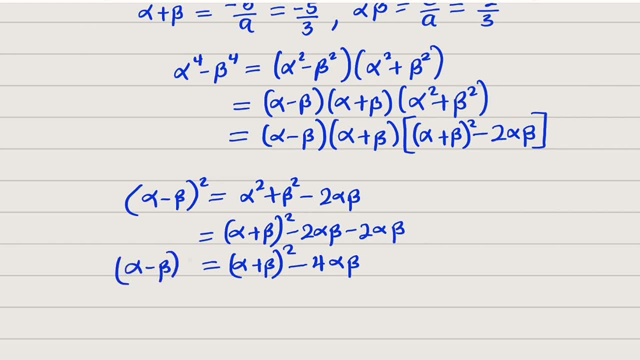 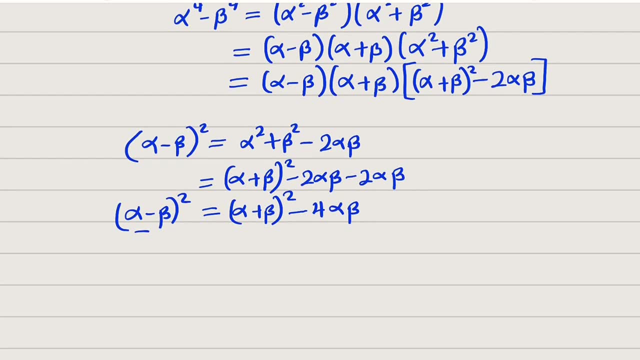 but remember, this is alpha minus beta all squared, but we are looking for alpha minus beta. therefore, we can take the square root of both sides. alpha minus beta will now be equal to plus or minus: the square root of alpha plus beta all squared, the minus for alpha beta. now, instead of this alpha minus beta, we can now write this: 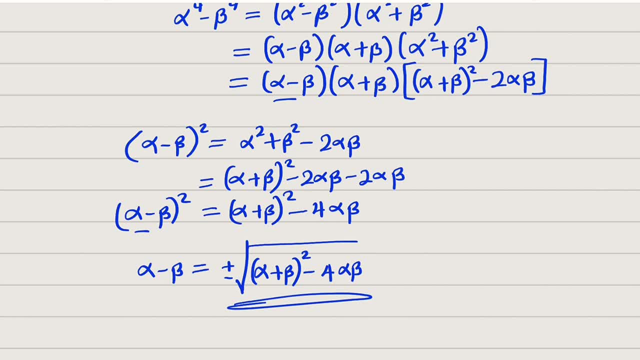 plus or minus square root of alpha plus beta squared minus 4 alpha beta. alpha Alpha to the power of 4 minus beta to the power of 4 is now equal to plus or minus the square root of alpha plus beta, or squared minus 4 alpha beta multiplied by alpha plus beta. 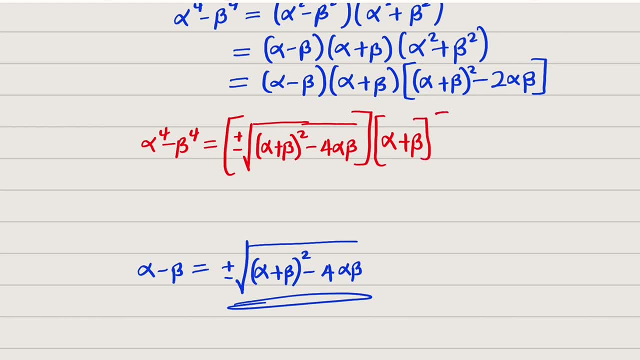 multiplied by again, alpha plus beta, raised to the power of 2 minus 2 alpha beta. all right, now everything is written in terms of product and sum of roots. now we can substitute our sum and the product in this equation, simplify to get our answer: alpha to. 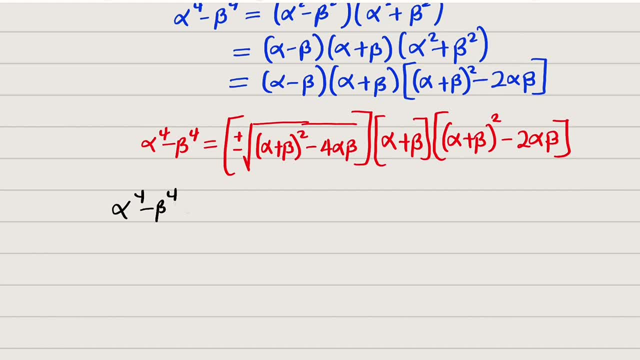 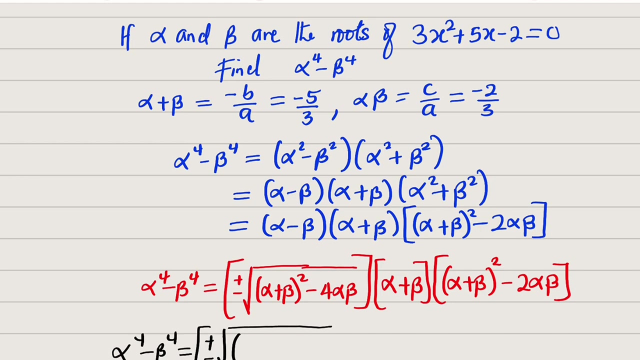 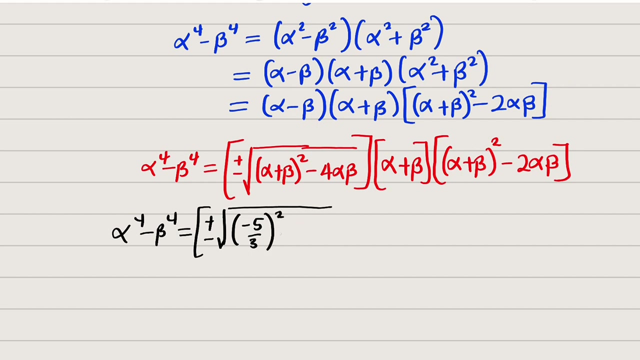 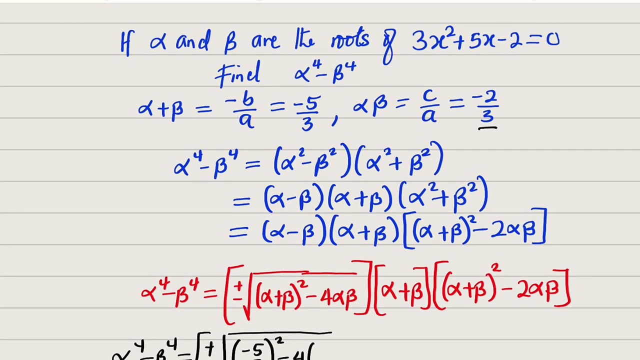 the power of 4 minus beta to the power of 4 is now equal to plus or minus into square root of the sum of roots, which is alpha plus beta. it is given as negative 5 over 3. so we have negative 5 over 3, but this one is squared minus 4 multiplied by the product. the product is negative 2 over 3. 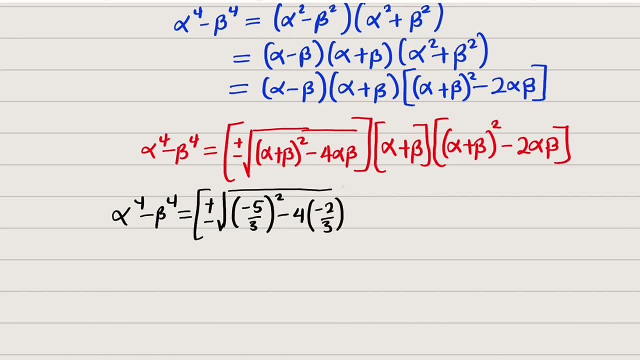 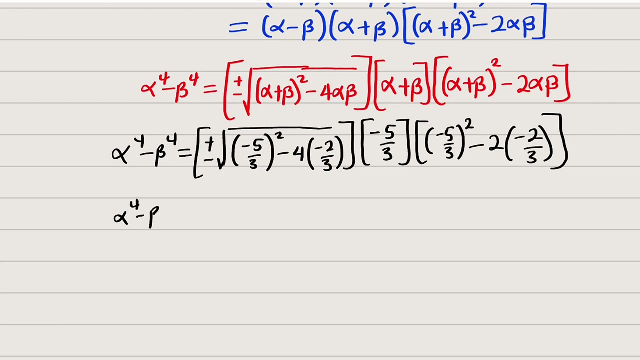 then multiply by this sum again, which is negative: 5 over 3. multiply by this sum again, which is negative: 5 over 3, all squared minus 2 multiplied by the product, which is negative, 2 over 3. now let us continue simplifying: alpha to the power of 4 minus beta to the power of 4 will be equal. 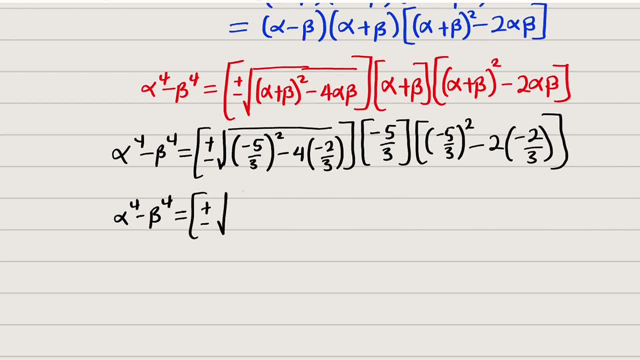 to plus or minus into the square root of negative. 5 squared is 25, 3 squared is 9. the minus minus is plus 4 times 2 is 8 divided by 3. multiplied by negative, 5 over 3 multiplied by negative, 5 squared is 25. divided by 3 squared is: 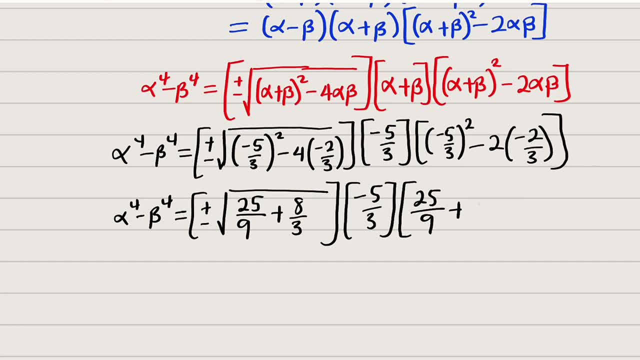 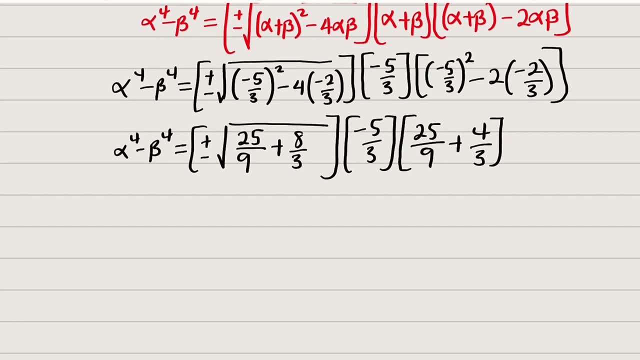 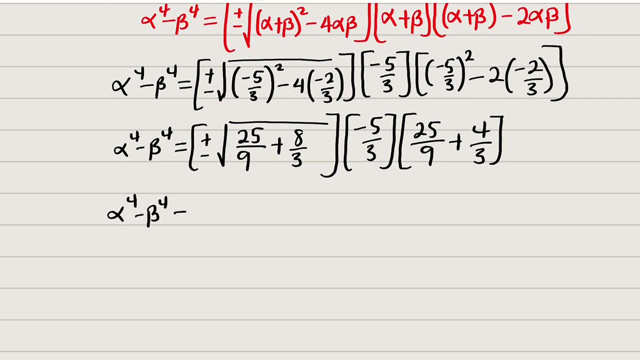 9 minus minus is plus. 2 multiplied by 2 is 4 divided by 3. we are moving alpha to the power of 4 minus beta to the power of 4 is now equal to plus minus, into the square root of now we can. 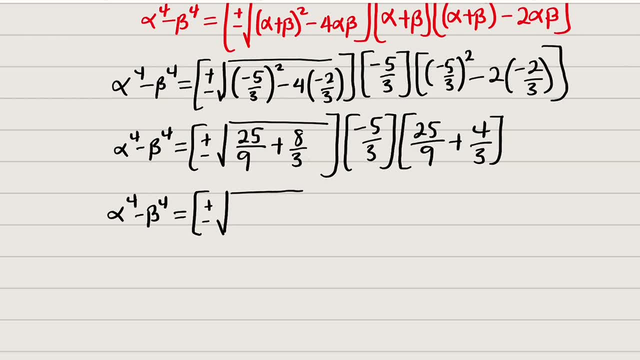 make this one to have a common denominator by multiplying this by 3. multiply this by 3 as well. we have 25 divided by 9, plus 24 divided by 9, multiplied by 3 is 15. it is equal to plus 26 divided by 9 plus 25 divided by 9. precise, 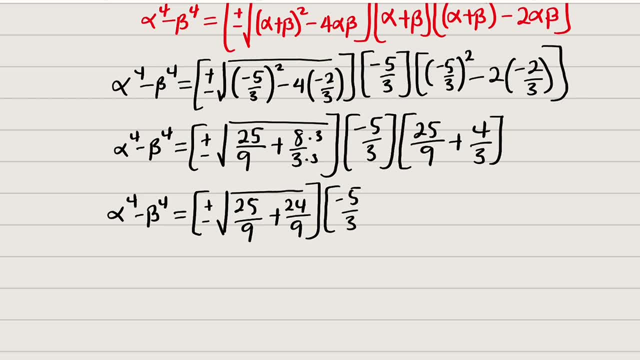 we counted 15 gaanemos. 15 of 5 is 25 divided by 9 plus 24 divided by 9 kişi, by negative 5 over 3 multiply by. we can do the same thing here: multiply the top and the bottom by 3. 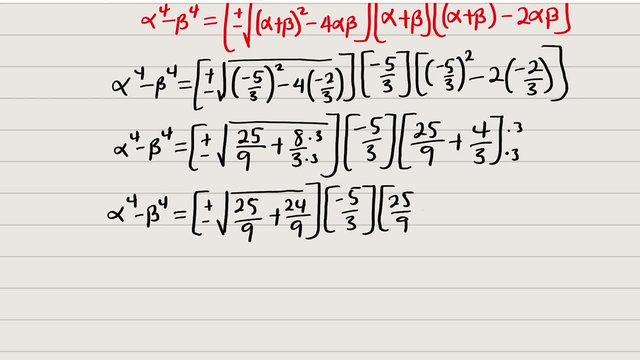 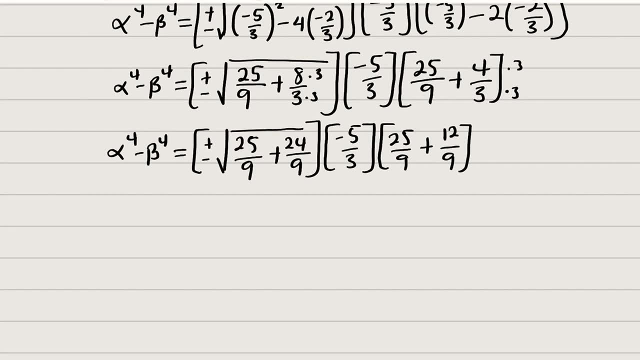 we have 25 over 9, plus 12 over 9. we are almost done. this is equal to plus or minus into square root of 49. divide by 9, multiply by negative, 5 over 3, multiply by this is going to be 37.